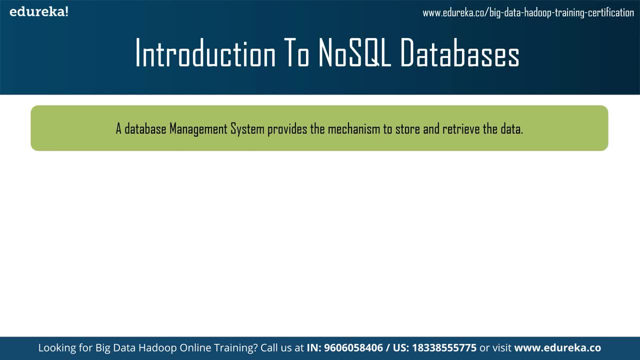 map. A database management system supports storage and manipulation of data, which makes data management easy. For example, an online telephone directory uses a database to store data of people, like phone numbers and other contact details that can be used by service provider to manage billing, client related issues and handle fall data, etc. So in simple words, we can say a database management system provides the mechanism to store data. 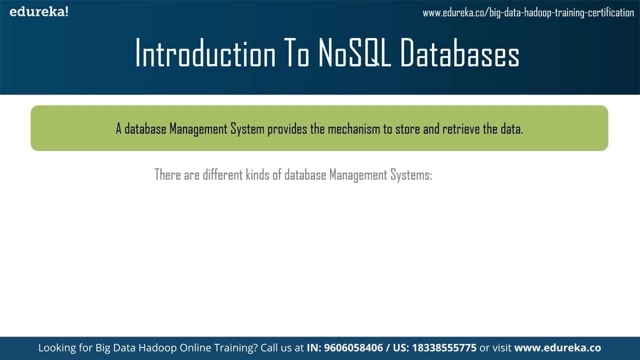 And retrieve the data. There are different kinds of database management systems present today, which are: relational database management system, known as RDBMS, online analytical processing, known as OLAP, and no sequel, which is popularly known as not only sequel. No sequel refers to all databases and data stores that are not based on the relational database management system or RDBMS principles. No sequel is a new set of 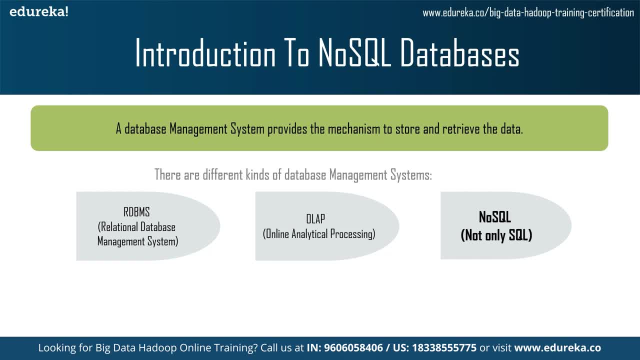 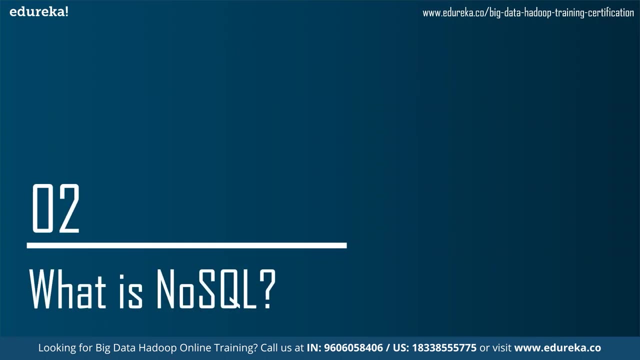 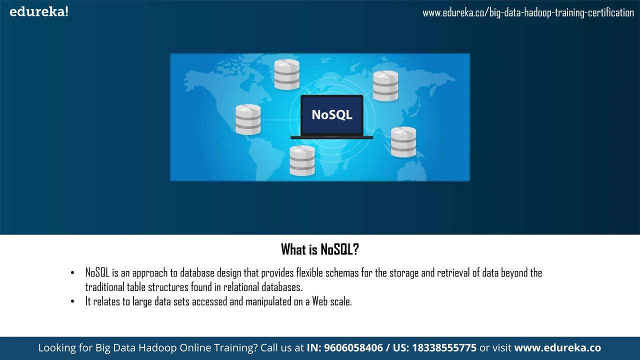 database that has emerged in the recent past as an alternative solution to relational databases. In 1998, Carl Strauss II introduced the term no sequel to name his file based database. So now we'll see what no sequel actually is. No sequel does not represent single product or technology, but it represents a group of products and various related data concepts for storage and management. 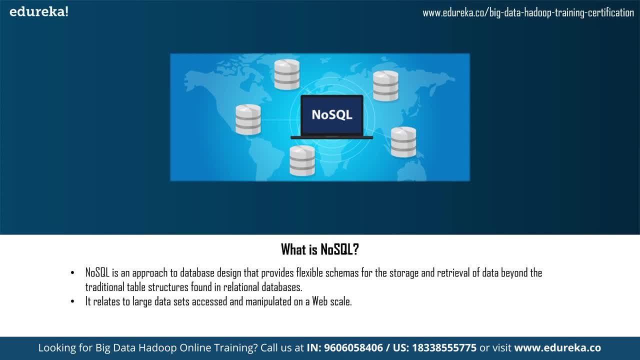 No sequel is an approach to database management that can accommodate a wide variety of data models, including key value, document, column and graph formats. A no sequel database generally means that it is non relational. It is distributed, flexible and scalable, So we can bind it up as an approach to database design that provides flexible schemas for the storage and retrieval of data beyond the traditional table structures found in relational databases. 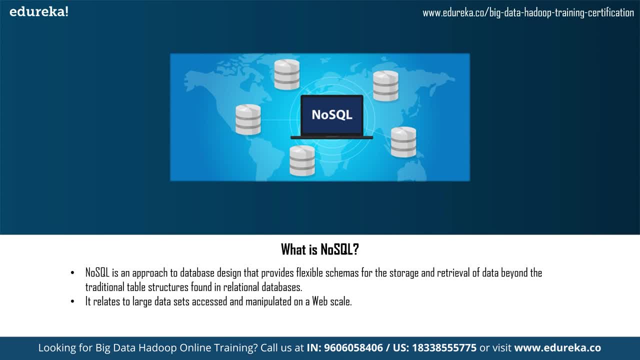 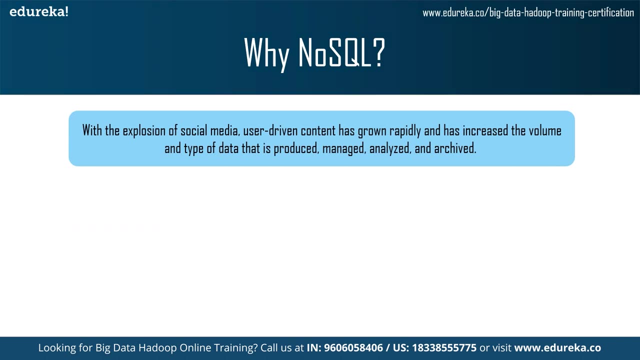 It relates to large data sets accessed and manipulated on a web scale. Now, when we have understood what is no sequel, the question arises is why to use no sequel. The concept of no sequel databases became popular with internet giants like Google, Facebook, Amazon, etc. Who deal with huge volumes of data. The system response time becomes slow when you use RDBMS for massive volumes of data. 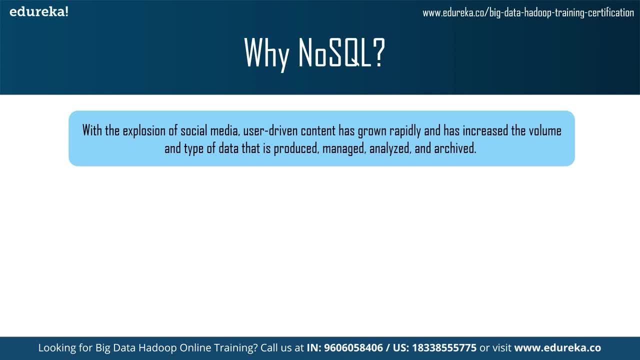 So to resolve this problem, we could scale up our systems by upgrading our existing hardware, But this process is expensive, So the alternative for this issue is to distribute database load on multiple hosts whenever the load increases. This method is known as scaling out. No sequel databases are non relational, So they scale out better than relational databases as they are designed with the web applications in mind. 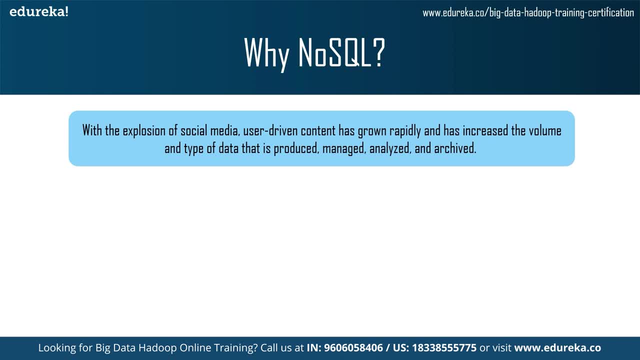 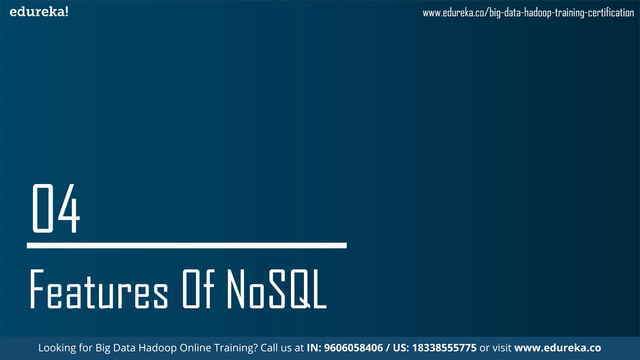 Now the no sequel database is exactly the type of database that can handle all sorts of semi-structured data, unstructured data, rapidly changing data or big data. So we can say, to resolve the problems related to large volume and semi-structured data, No sequel databases have emerged. Now let's talk about the features of no sequel databases. No sequel databases never follow the relational model and don't provide 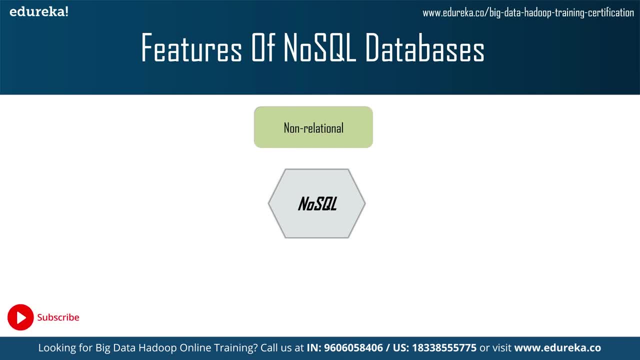 tables with flat, fixed column records, So they doesn't require object oriented mapping and data normalization. Most of the no sequel databases are open source. Multiple no sequel databases can be executed in a distributed fashion, and they offer auto scaling and fail over capabilities. They follow shared nothing architecture, which enables less coordination and higher distribution. No sequel databases are: 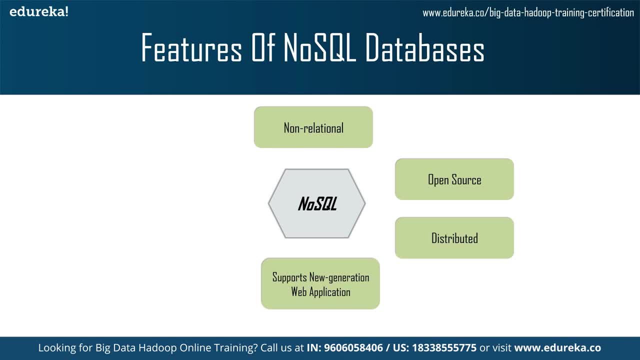 non relational and offer heterogeneous structures of data in the same domain, which supports new generation web applications. No sequel databases are either schema free or have relaxed schemas and do not require any sort of definition of the schema of the data. And no sequel databases offer easy to use interfaces for storage and querying data provided and APIs allow low level data manipulation and selection methods. 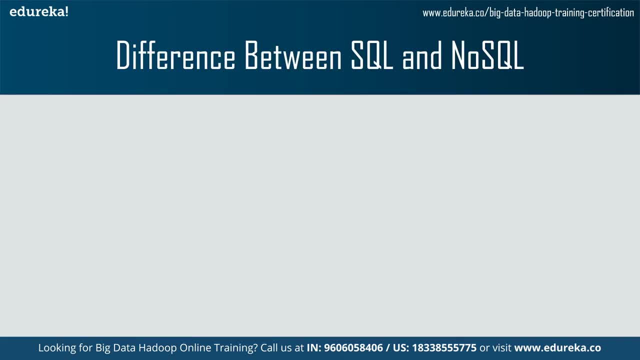 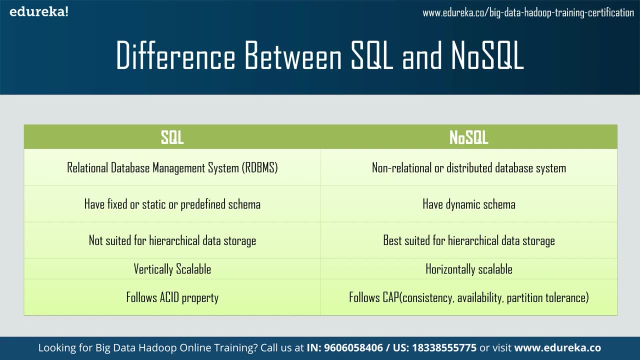 Now we can compare SQL and no sequel. On comparing SQL and no sequel, we can find the differences like: SQL databases have fixed or static or predefined schema, while no sequel databases have dynamic. already Sequel databases are not suited for hierarchical data storage, while no sequel databases are best suited for hierarchical data storage. 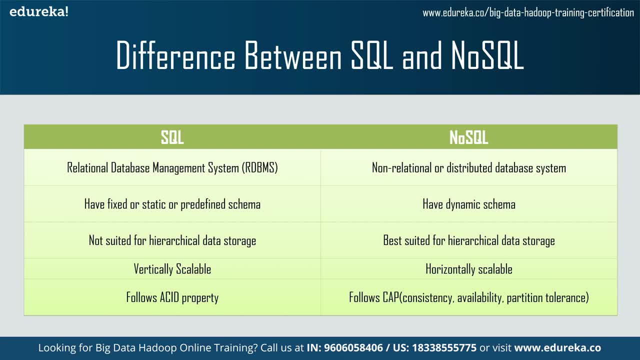 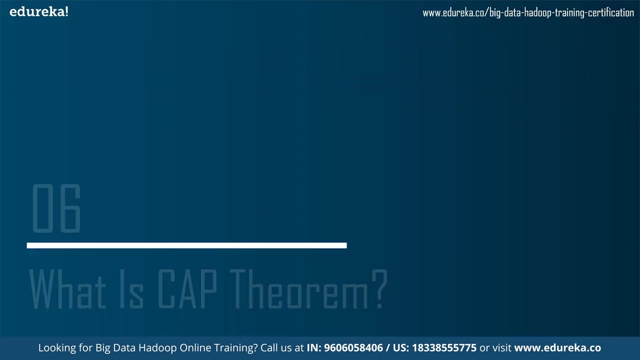 Sequel databases are vertically scalable- tastelessly. Now NoSQL databases are horizontally scalable as they are distributed. sequel databases follow acid property, that is atomicity, consistency, isolation and durability, while NoSQL databases follow cap theorem, that is consistency, availability and partition tolerance. now you must be wondering. 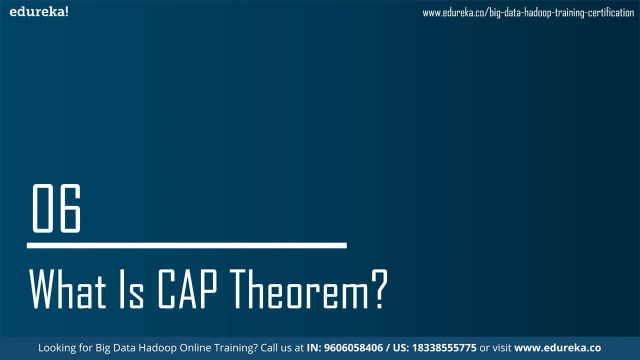 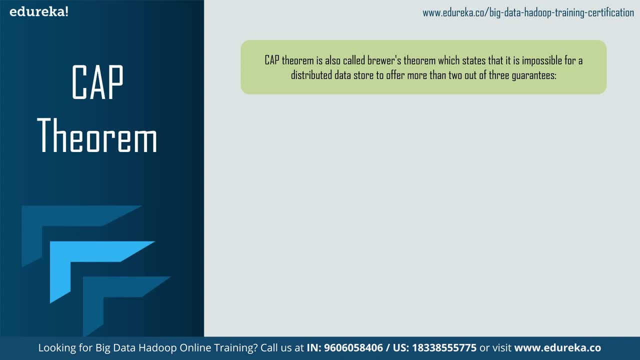 what is cap theorem, which plays an important role in NoSQL databases. cap theorem is also called Brewer's theorem and it states that it is impossible for a distributed data store to offer more than two out of three guarantees, which are consistency, availability and partition tolerance. so, basically, some NoSQL databases offer consistency and partition tolerance, while some offer availability. 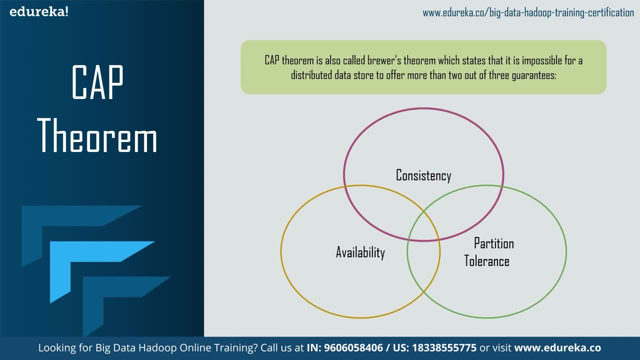 and partition tolerance. but partition tolerance is common. as NoSQL databases are distributed in nature. based on the requirement, we can choose which NoSQL database has to be used. different types of NoSQL databases are available based on the data models. so before talking about those, let's just understand. 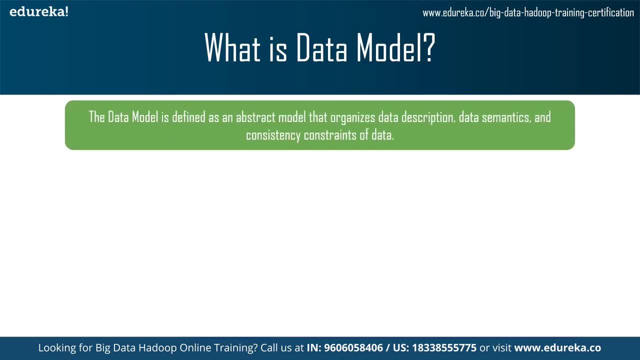 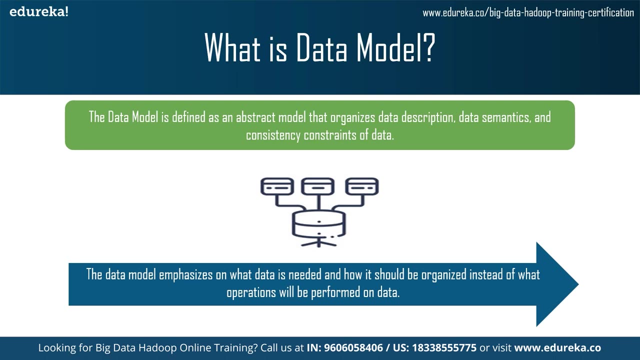 what is data model? the data model is defined as an abstract model that organizes data description, data semantics and consistency constraints of data. the data model emphasizes on what data is needed and how it should be organized, instead of what operations will be performed on data. now we can see. 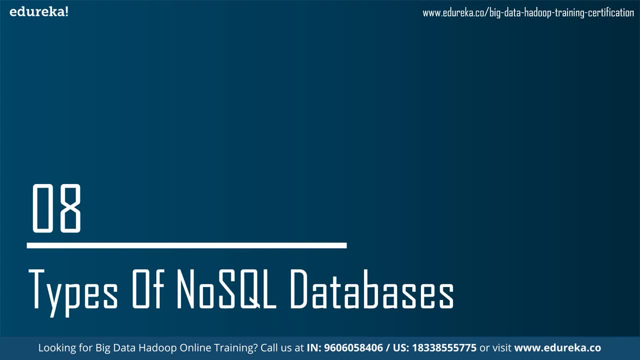 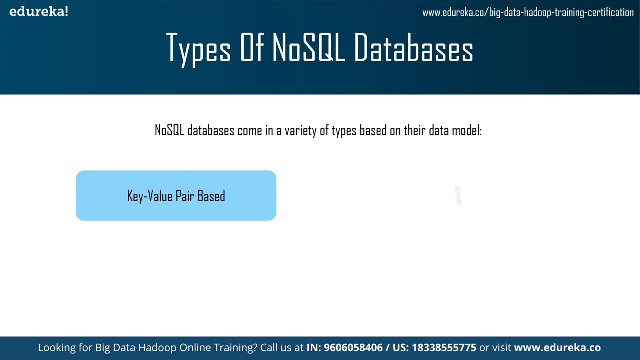 the types of NoSQL databases available, based on their data models. so NoSQL databases come in a variety of types, which are key value pair based, graph based, column based and document based. now we will see each of these NoSQL databases one by one. so let's start with key value pair based NoSQL databases. 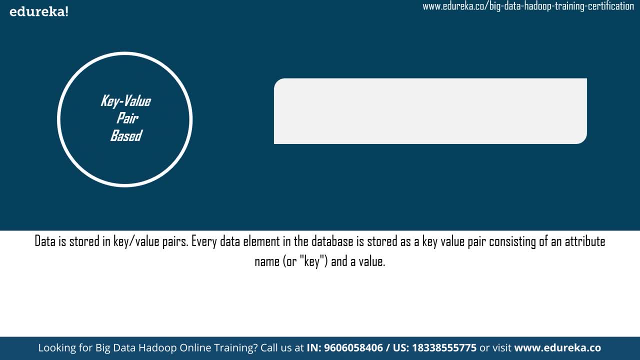 databases. in this data is stored in key-value pairs. each data element in the database is stored as a key-value pair consisting of an attribute, name or key and a value. these databases are used to handle lots of data and heavy load. some of key-value pair based NoSQL databases include Redis: 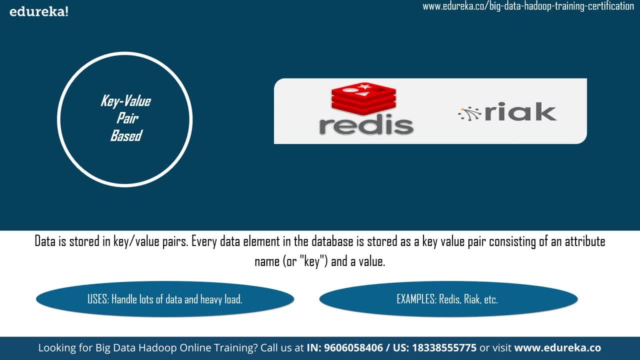 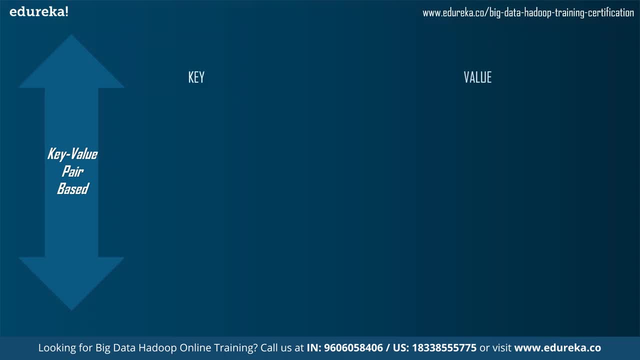 react, Voldemort, Etc. Now we will see a demo for key-value pair based NoSQL databases. Data has to be stored as key-value pairs, So here our key is name and value, for this key is Richard, So it makes a pair of key and value. that is actually the data. similarly, 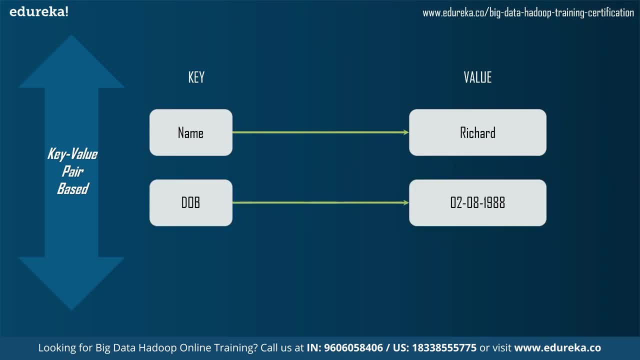 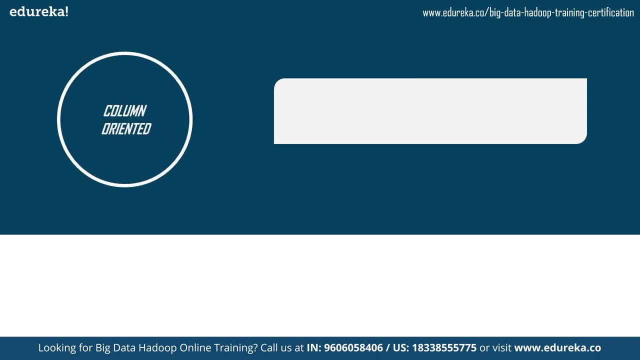 for dob key 2nd August 1988 is the value and for address key 32 W, NYC is the value. now moving on, let's understand column-oriented NoSQL databases. column-oriented databases work on columns, Where each column is treated separately and the values of single column databases are stored contiguously. these databases 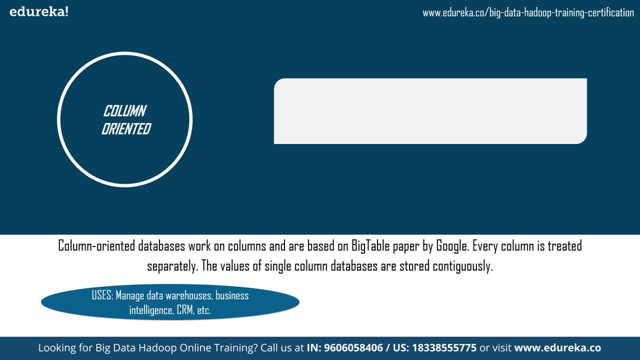 are used to manage data warehouses, business intelligence, CRM, library, card catalogs, etc. Some of column-oriented NoSQL databases include HBase, Cassandra, etc. And these databases are based on big table paper by Google. Now let's understand this with a demo. 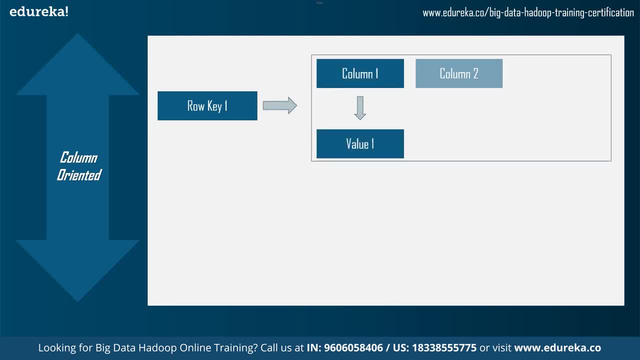 We have row keys. They are associated with the columns. So here we have a row key 1, associated to column 1, which has value 1, and the column 2, which has value 2, and column 3, which has value 3.. 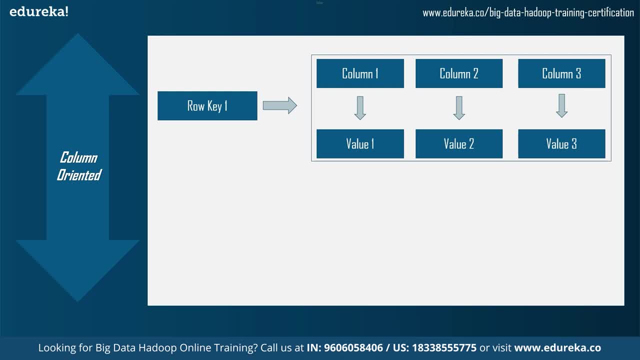 We can see, k1 is associated to three columns where each column has some value. Similarly, row key 2 is associated to column 1 and column 2, which have value 1 and value 2 respectively. here row keys are for grouping the columns. 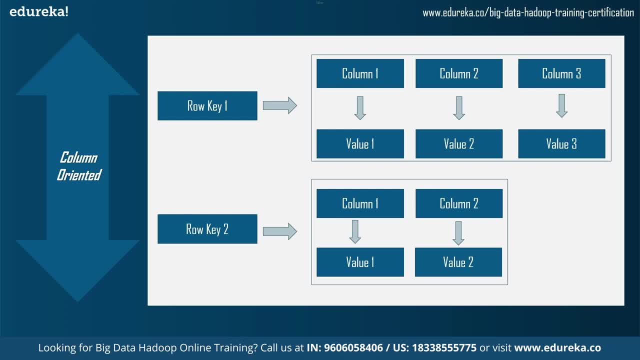 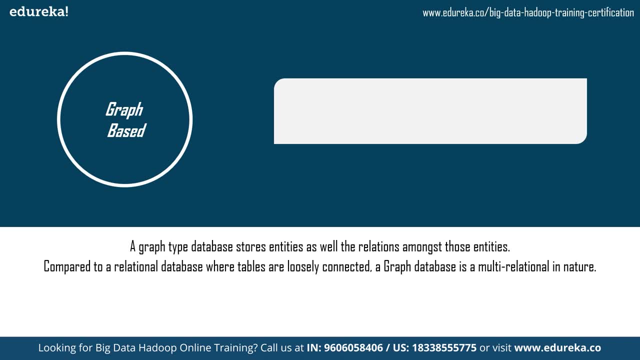 but actual data is stored in the columns. now, moving on, Let's understand the graph based databases and graph type database stores entities as well as the relations amongst those entities, the entities stored as a node with the relationship as edges, and edge gives a relationship between nodes, and every node and edge have a unique identifier, a graph database. 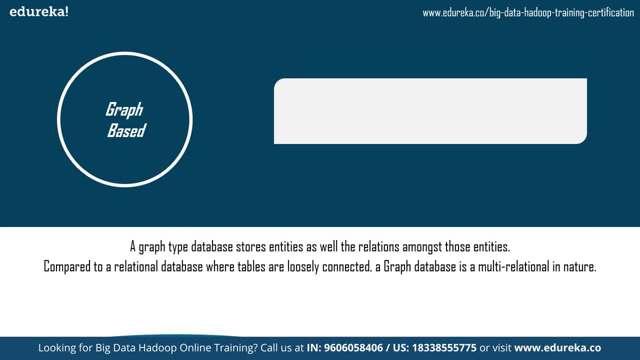 is a schema, less yet multi-relational in nature. These databases are used to manage social networks, logistics and spatial data. some of graph based no sequel databases include Neo4j, orient, DB, Etc. Now let's understand graph based databases with the demo. 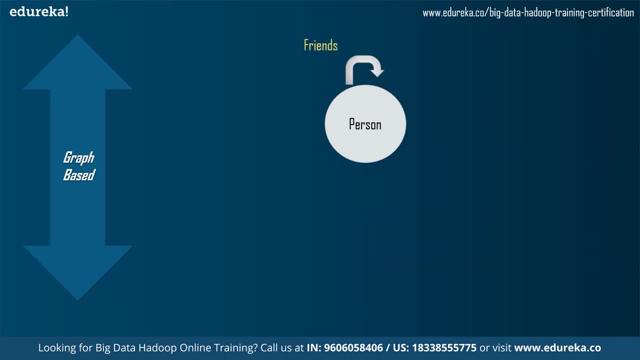 We have a person as node who has a relationship with another person as friend and he has other relationships with City that he lives in. a city whose properties could be address as a node can have multiple relationships and properties. here the person has one more relationship with the city that he likes. the city and properties include the ratings. 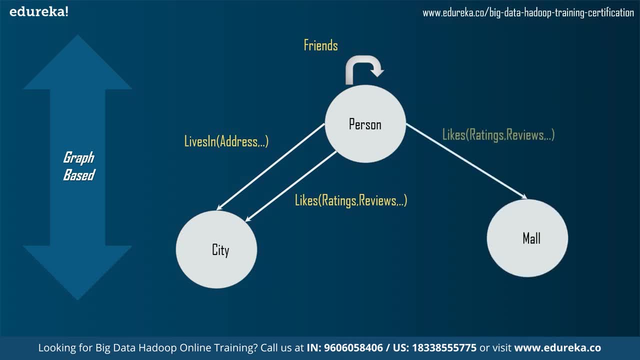 and reviews. similarly, the person likes a mall based on the properties, like ratings and reviews, and the node mall has a relationship with the city that it is located in- a city and properties include address. So we can infer that in graph based databases the data is stored. 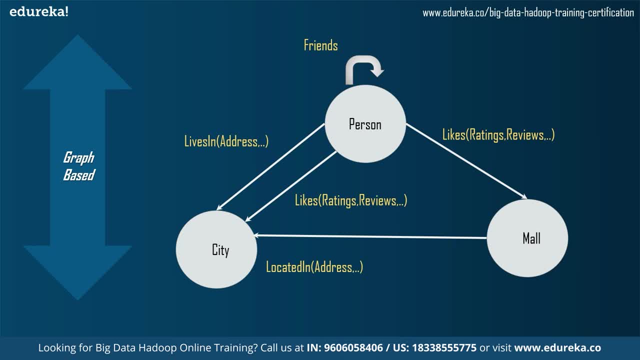 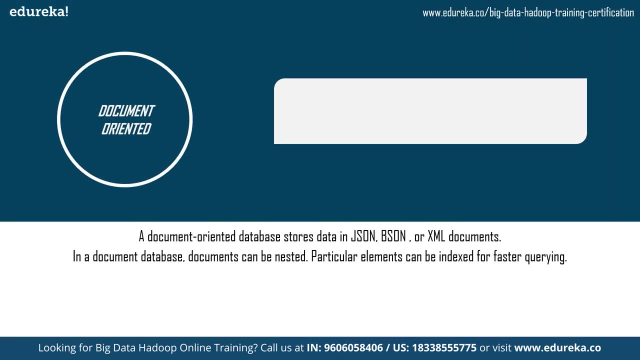 as nodes, relationships and properties, Where properties can be of nodes as well as of relationships. now, moving further, Let's understand document oriented, no sequel databases. a document database stores data in Jason Beeson and XML documents. in a document database, documents can be nested and particular elements can be indexed for faster querying document databases. 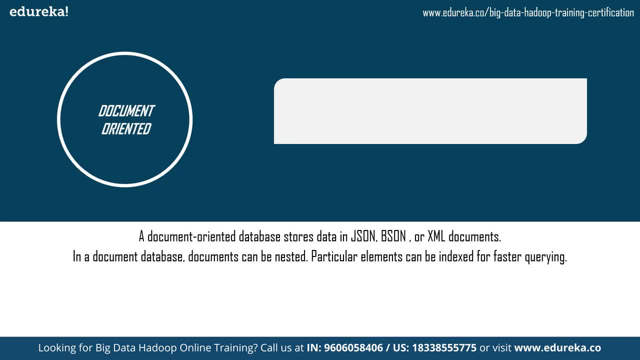 make it easier for developers to store and query data in a database by using the same document model format they use in their application code. These databases are used for the applications having dynamic schema and characteristics. some of document oriented no sequel databases include MongoDB, couch base, Etc, and MongoDB is the most popular database in no sequel databases. 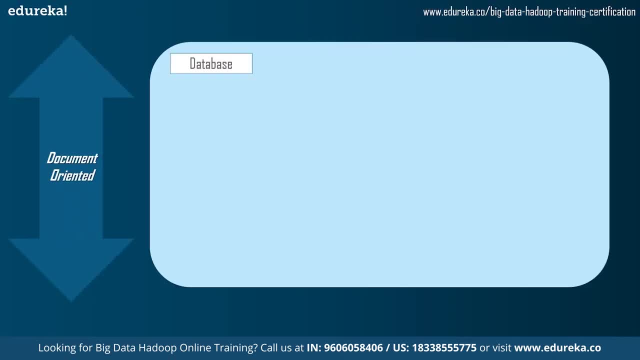 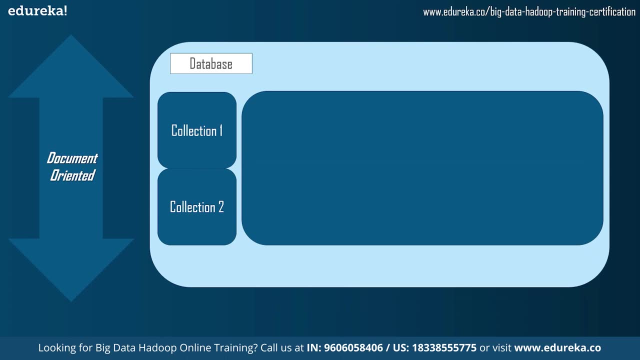 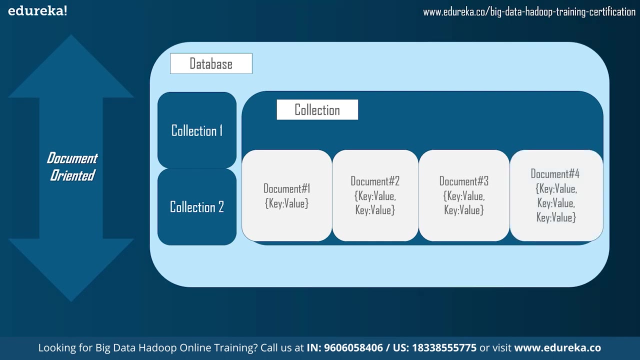 Now let's understand this with the demo. So we have a particular database which can have multiple collections. Here we have collection 1 and collection 2.. Let's see how collection is made. each collection can have multiple documents with different schemas, as it has dynamic schema. 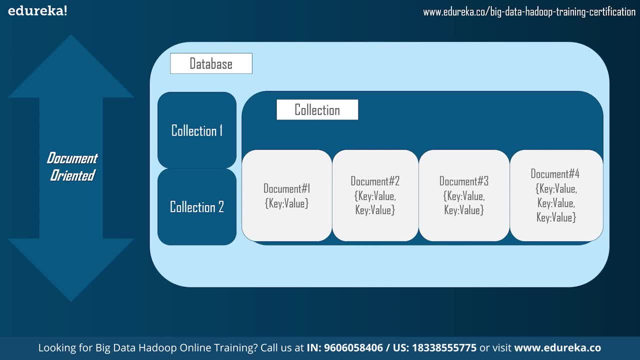 So here we have document 1 with V 1 key value pair, then document 2 with 2 key value pairs, document 3, again with 2 key value pairs and finally document 4 with 3 key value pairs. These key value pairs can be of any type.